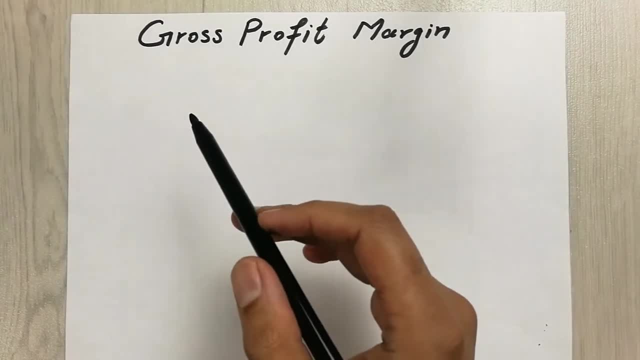 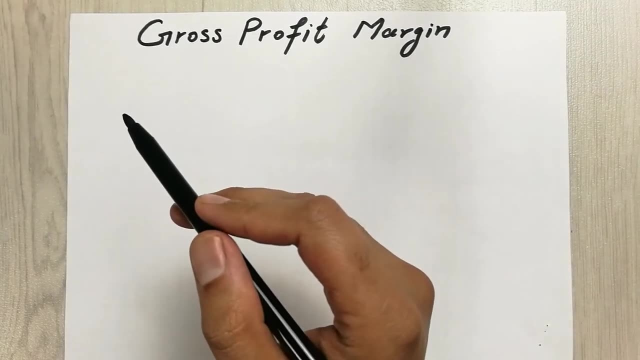 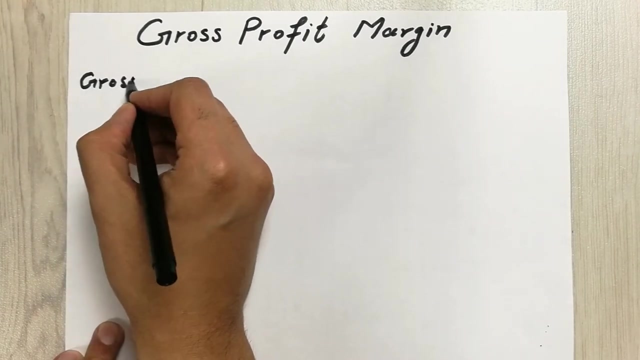 Hello, guys, I hope you are doing really, really well. Today I am going to show you how to calculate the gross profit and gross profit margin. So in the first step we will write the formula for gross profit. So, guys, gross profit equals to sales revenue. Okay, so gross profit equals to: 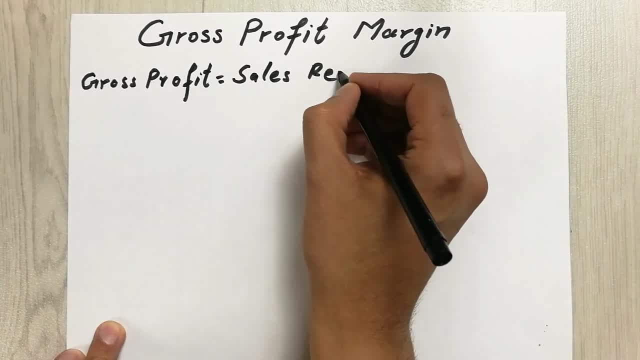 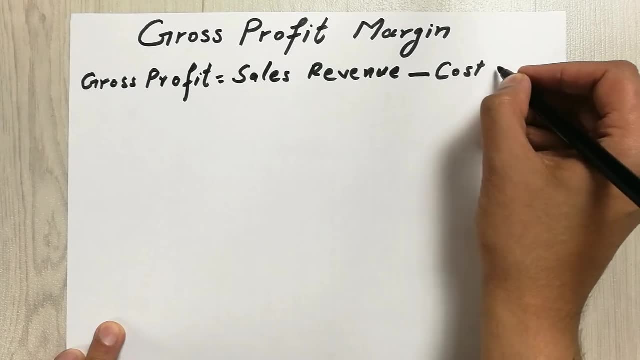 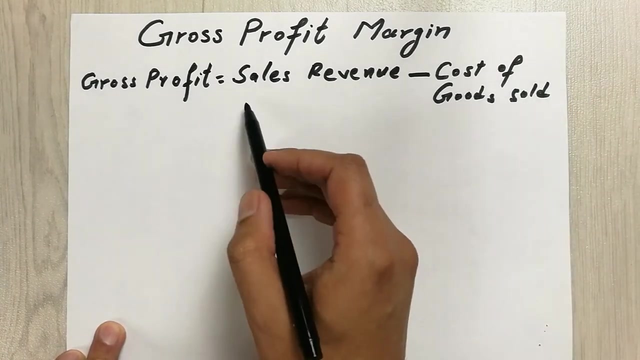 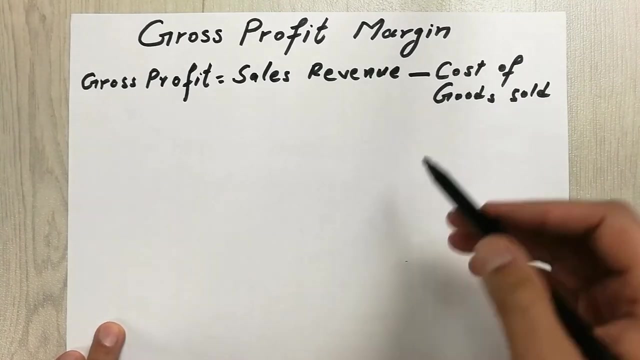 sales revenue: Okay, minus cost of goods sold. So cost of goods sold: Okay. so, guys, sales revenue is the total sales that is generated. Okay, so this is very simple. And cost of goods sold is the direct cost of producing. 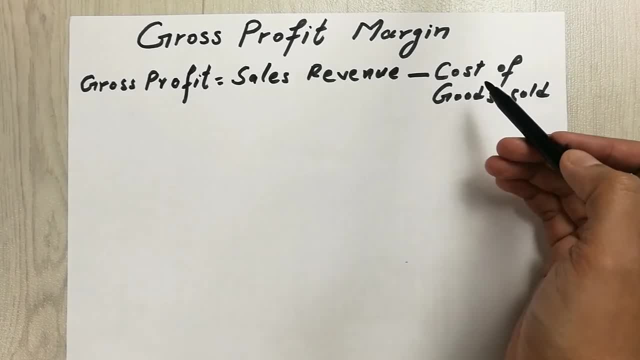 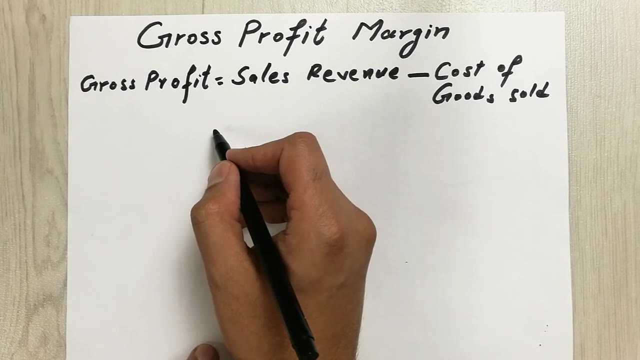 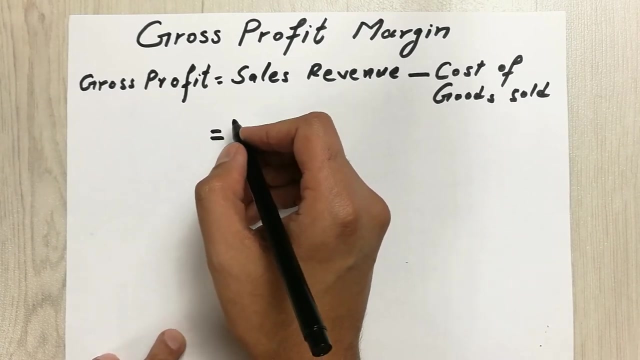 The goods. So it includes, for example, the cost of material and labor. So whatever cost that is required to produce that good is called cost of goods. Okay, so now in the next step we will put the numbers, So our sales revenue. let's say it is 35,000.. Okay, dollars or rupees. 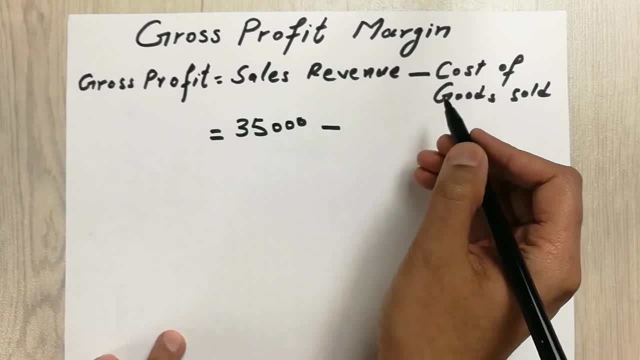 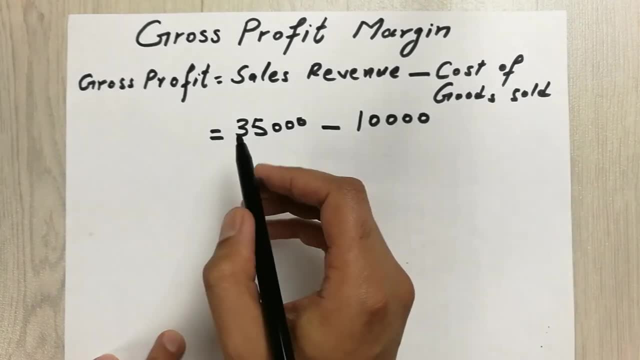 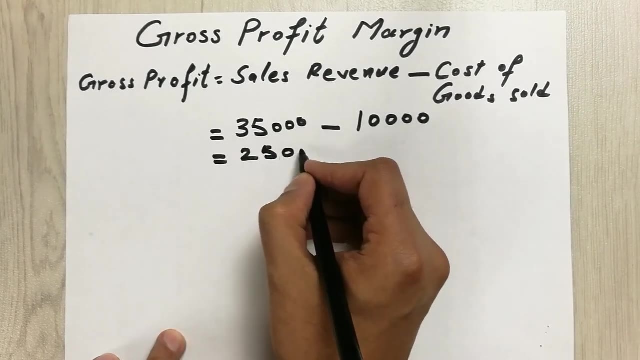 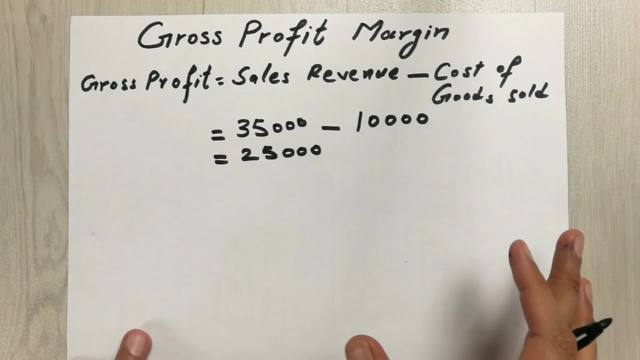 or whatever currency you want, And our cost of goods sold is 10,000.. Okay, So 35,000 minus 10,000.. Our answer will be 25,000.. Okay, so this is the gross profit. So now we will move to the next step. 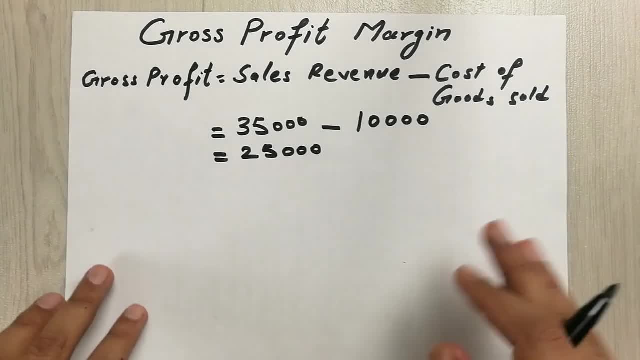 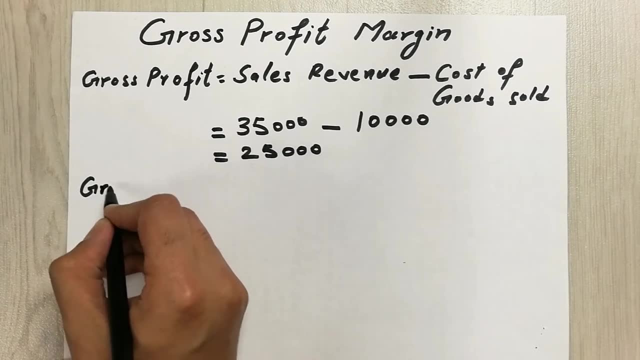 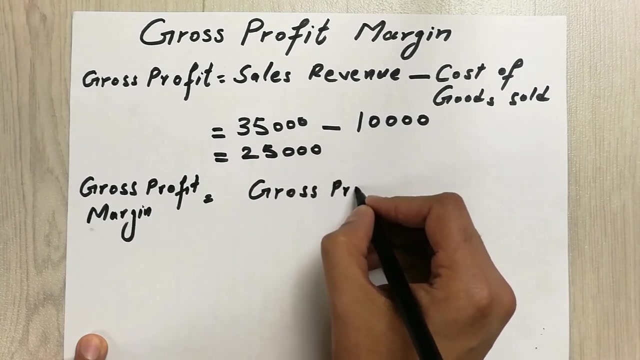 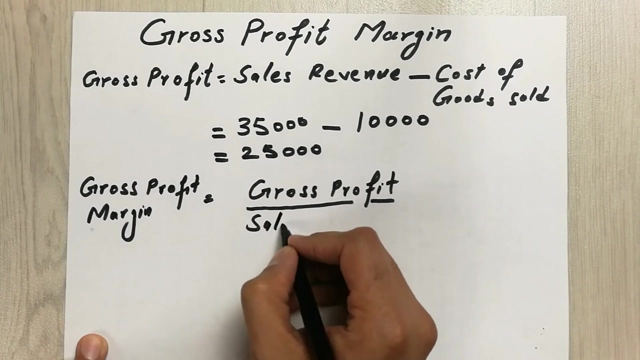 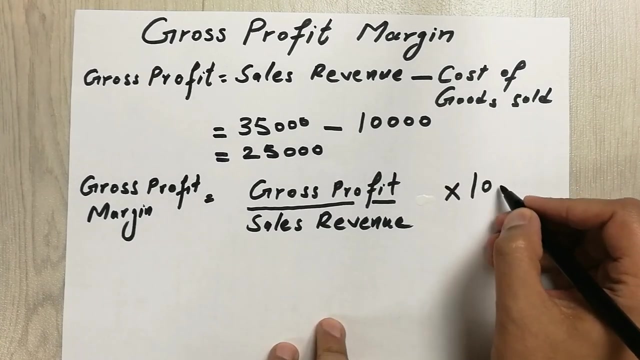 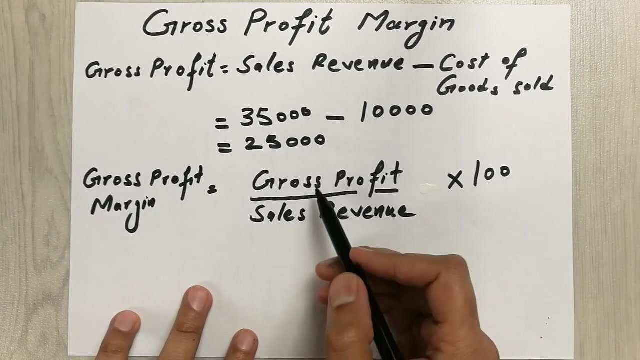 which is gross profit margin. So, guys, gross profit margin, we show it always as a percentage. So formula for gross profit margin is: gross profit, Okay, Divided by sales revenue, Purchase demand Multiplied with 100.. Okay, so now we will put the figures over here. So, gross profit, we're already.